In today's video, we're going to look at how we can find the original value of something after it's already changed by a certain percentage, and we sometimes call this reverse percentages. For example, let's take this question where we're told that the price of a house has 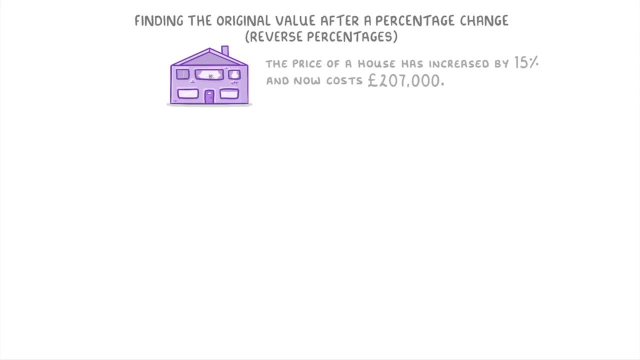 increased by 15% and now costs £207,000, and we're being asked to find out what the original price must have been. So, in this scenario, the £207,000 is the new price, after some original price which we don't know yet has been increased by 15%. 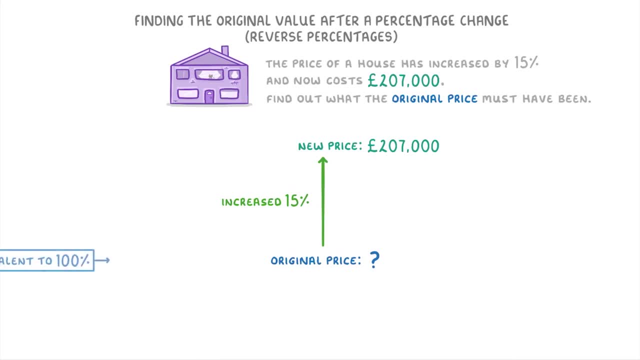 The best way to think about these questions is to remember that the original price is always equivalent to £100,000.. So in this example, where the price has increased by 15%, the new price is effectively 115%, because we can think of it as the original 100% plus the extra 15%, which is 115% in. 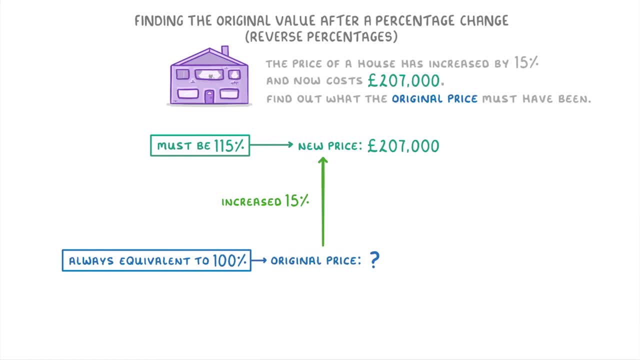 total. This way of doing it is actually really helpful, because it means that we can find out what 1% is by dividing the £207,000 by 115, to get £1,800.. And because £1,800 represents 1%, all we have to do to find the original price, which. 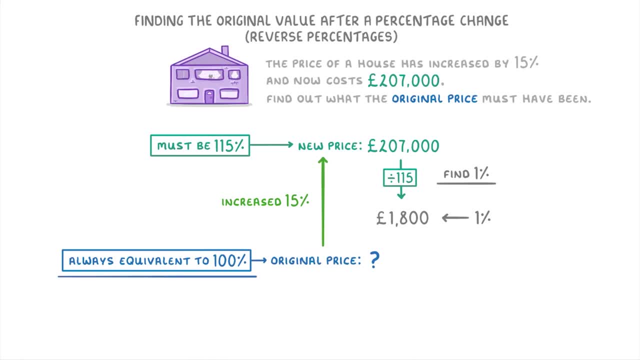 remember we said earlier was: 100% is multiply £1,800 by 100, showing us that the original price was £180,000.. Now this here is a little bit messy and potentially a bit confusing, so you don't really want to lay out your workings like this in the exam. 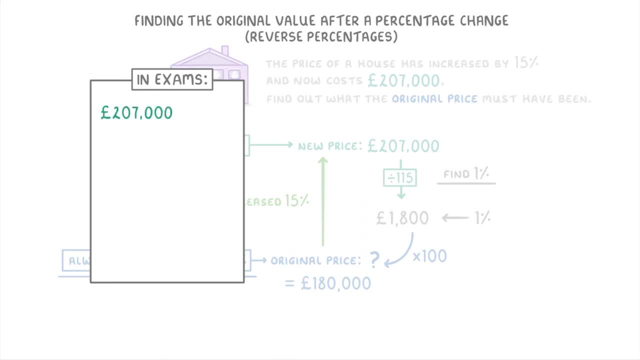 Instead, you want to first of all think of the £207,000 as equivalent to 115% of the original value. So if we want to find the original value, which is 100%, we first need to find 1% by dividing the £207,000 by 115, which is £1,800. 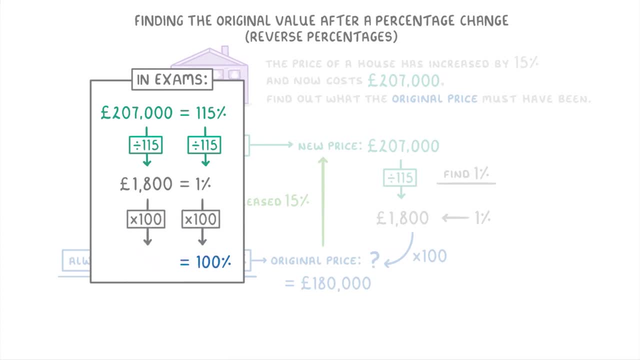 And then we can multiply that by 100 to show that the original price was £180,000.. So, basically, this technique- and in fact every example that we're going to look at in this video- is all about finding out the value of 1%. 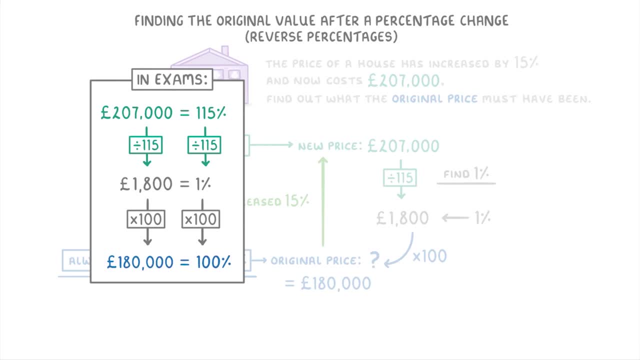 And once you find out what 1% is worth, you can use that to find out the value of any percentage that you want. And this way of doing it, in the box here, is basically the simplest way of showing your workings, And this is how I would write this question in the exams. 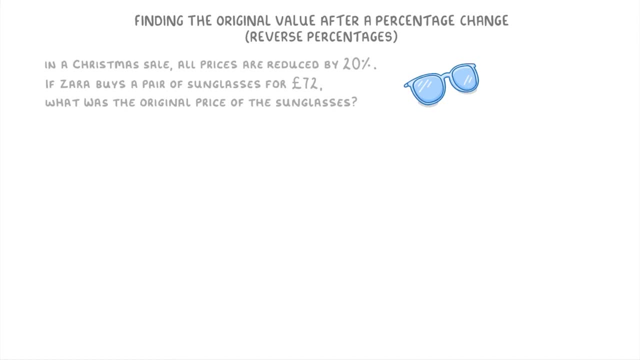 Let's try doing this for another one. In a Christmas sale, all the prices have been reduced by 20%. If Zara buys a pair of sunglasses for £72, what was the original price of the sunglasses? So in this question we're looking for the original price before it was discounted. 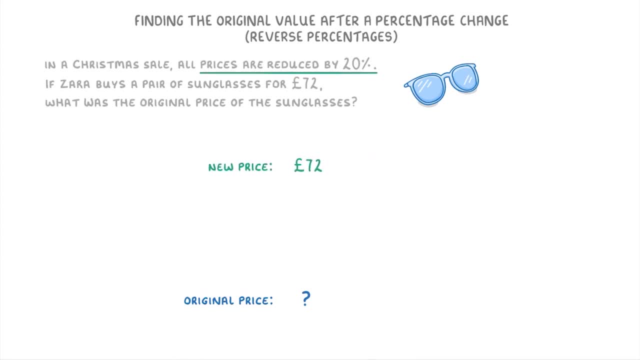 And we know that once it's been reduced by 20%, the new price is £72.. Just like before, we can think of the original price as £100.. So if it's been reduced by 20%, then the new price for sale must be 80%. 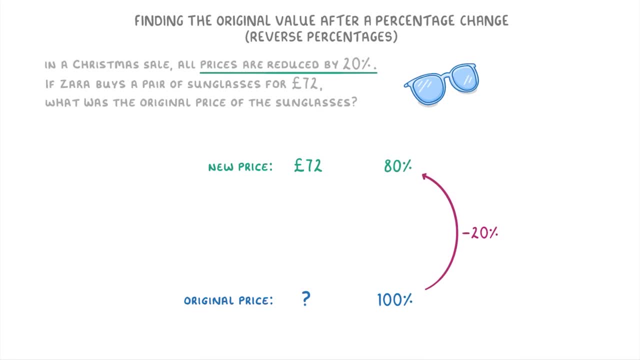 Because 100 minus 20 is 80. So we now know that 72 £ is equivalent to 80%, and this means that to find 1%, we just have to divide 72 by 80 to get 0.9 £. 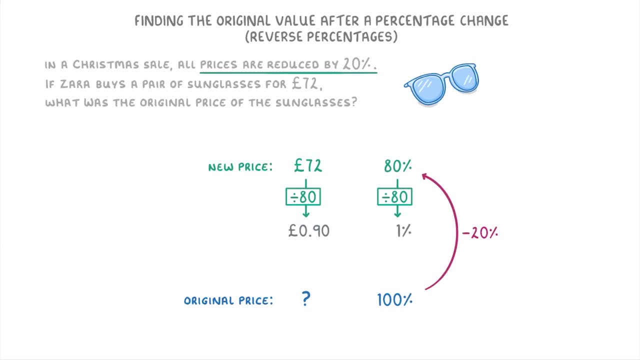 And to find the original price, we just multiply this 0.9.. Which is 1000. That's also a degree- by 100 to get £90. So the sunglasses must have cost £90 before the sale. Okay, so for this one it says that the value of a car decreased by 8% in the first year. 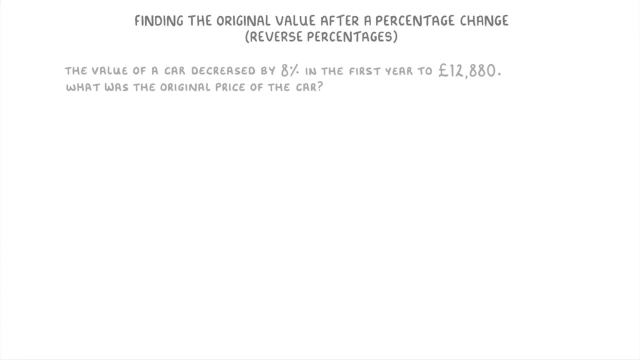 to £12,880.. What was the original price of the car? Well, this time £12,880 is a new price and we know that it's decreased by 8% from the original price, which we don't know the exact value of, but we can think of as 100%. 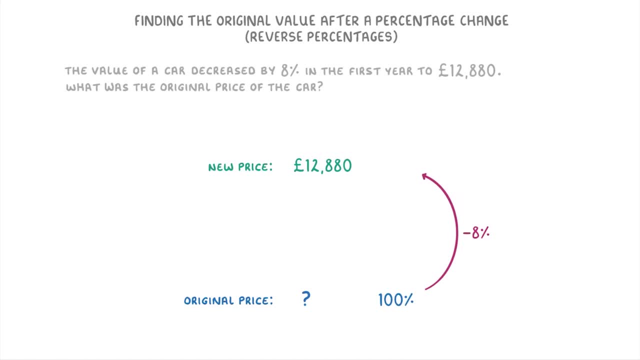 This means that the new price must be 100 minus 8, or 92% of the original. So we're going to have to do £12,880 divided by 92 to find that 1% is £140, and then we can multiply that by 100 to find that the original 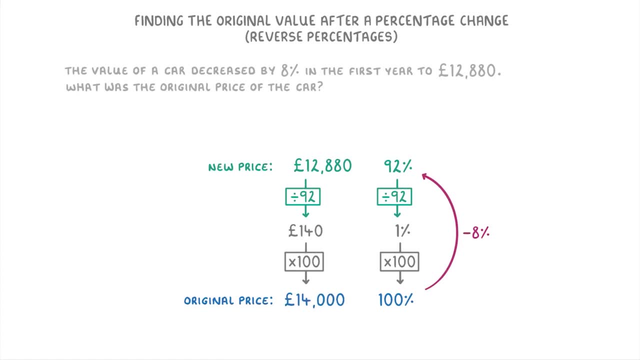 price must have been £14,000.. Now, just before we finish, we need to look at a slightly different version of these reverse percentage questions, which are ones where they tell you how much the price has changed by rather than telling you the new price. For example, in this question here, we're told that 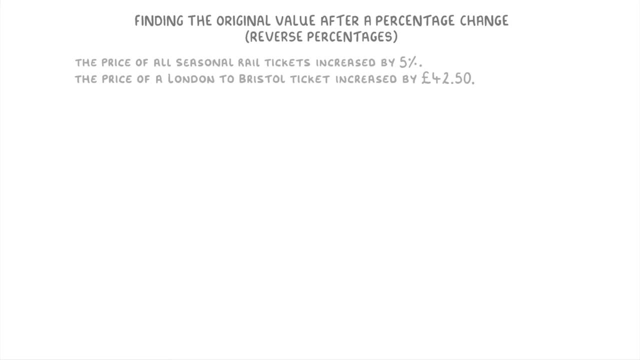 the price of all seasonal rail tickets increased by 5% and that the price of the London to Bristol ticket increased by 5%. So we're told that the price of all seasonal rail tickets increased by 5% and that the price of the London to Bristol ticket increased by 5%, increased by £42.50.. 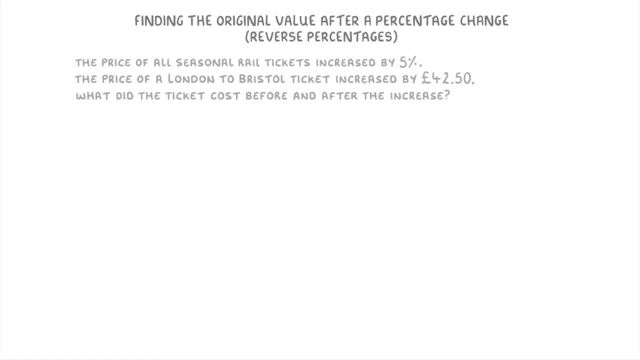 What did the ticket cost before and after the increase? So, just like before, let's think of it in terms of the original price, which is 100%, and a new price, But this time it's a bit different, because we don't know the. 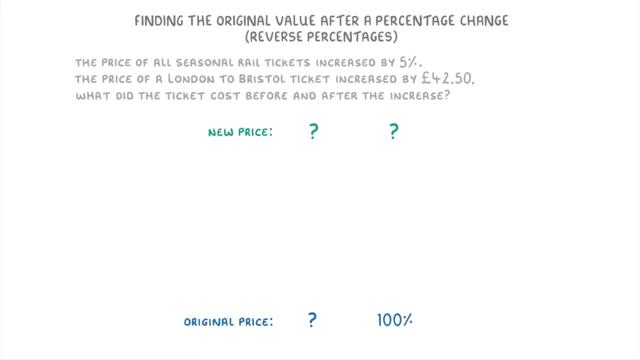 value of the new price. Instead, we're given extra details about the change in price. The question tells us that the price has increased by 5% and that the actual value of that 5% increase is £42.50.. So this time to find 1%, like we've been doing for the other. 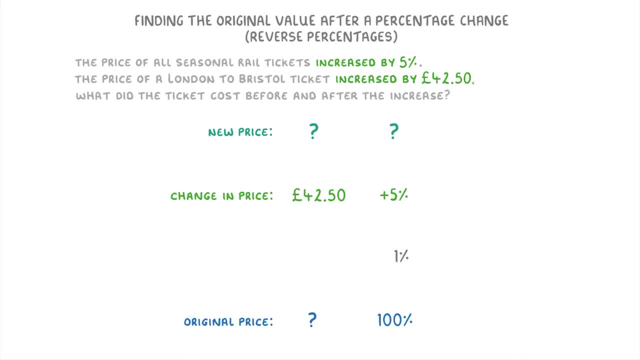 questions. we need to divide the £42.50 by 5, to find that 1% is £8.50. And so now to work out the original price, we can just multiply the £8.50 by 100 to get £850.. So the seasonal ticket cost. 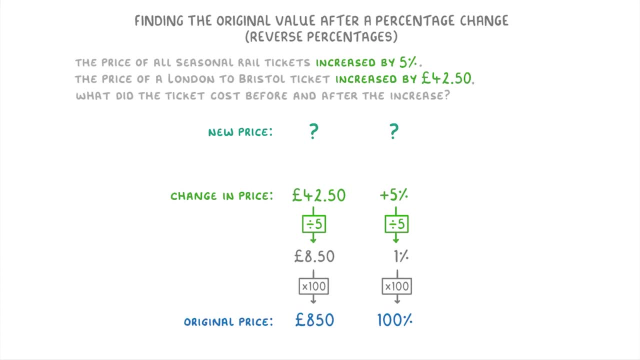 £850 before the price increase. Then to find the new price after the increase, we just multiply £8.50 by 105, because we want the original 100% plus the extra 5%, which gives us 105%. So that will be £892.50.. 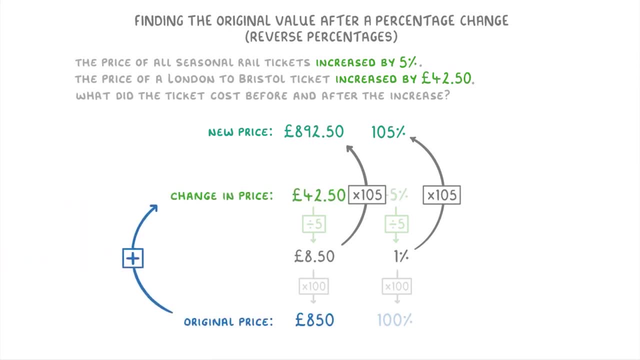 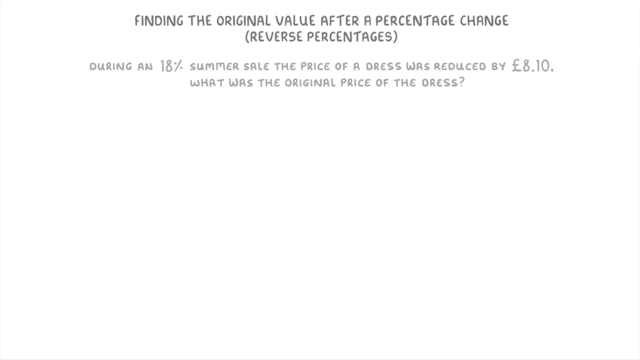 Or, alternatively, you could have also just added the original price of £850 to the change in price of £42.50, and that would have also given us £850.. So either way of doing it is perfectly fine. Let's try one more of this type. During an 18% summer sale, the price of a dress was reduced by